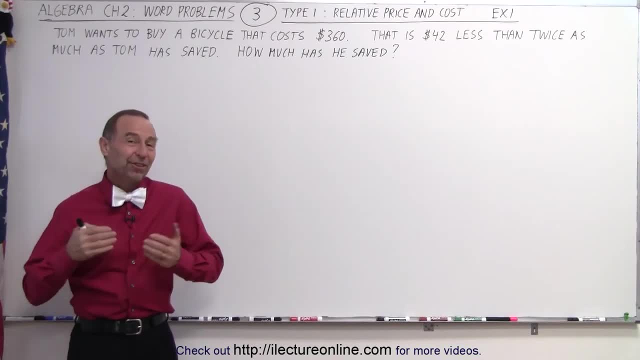 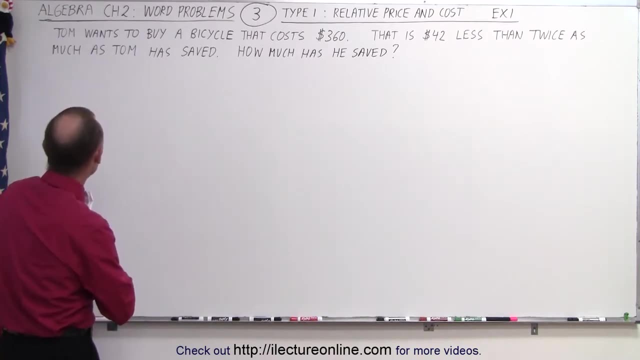 Welcome to iLecture Online. Here's the first example of the first type of word problem: word problems dealing with relative price and cost. The problem reads as follows: Tom wants to buy a bicycle that costs $360,, that is, $42, less than twice as much as Tom has. 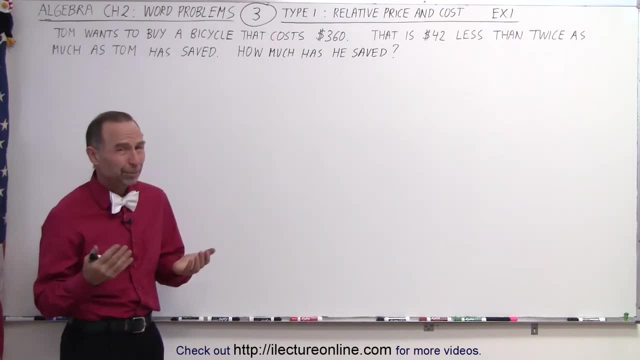 saved. How much has he saved? Well, how do we start a problem like that? Typically, it starts with the sentence: let X equal something. So let's start with that: Let X equal. Now we need to let X equal something, And in this case, we probably want to let X be the unknown. 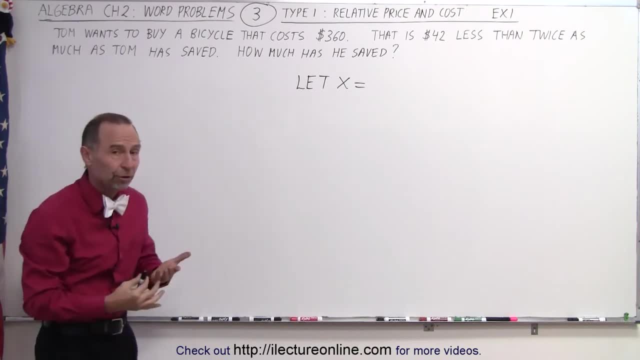 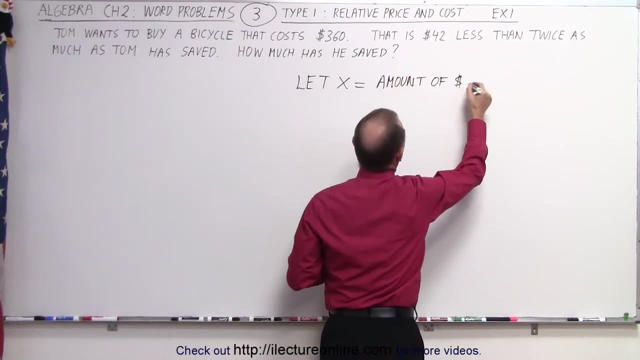 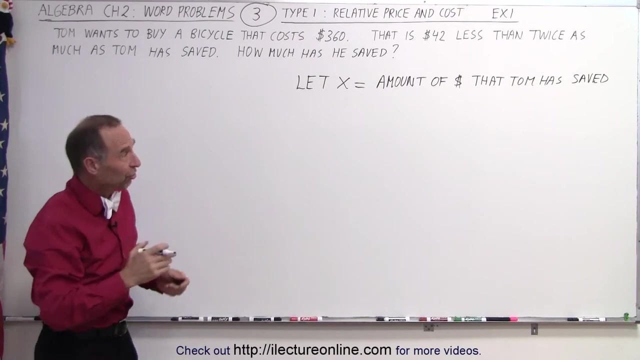 how much Tom has saved, because everything is in terms of how much he has saved. So let X equal represent the amount of dollars that Tom has saved. Notice how that statement is fairly descriptive. It says exactly what it means: that X represents the amount of dollars, the amount of money that Tom has saved. Don't say let X equals Tom or something. 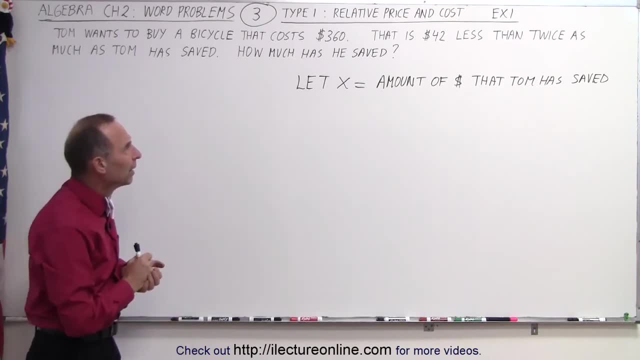 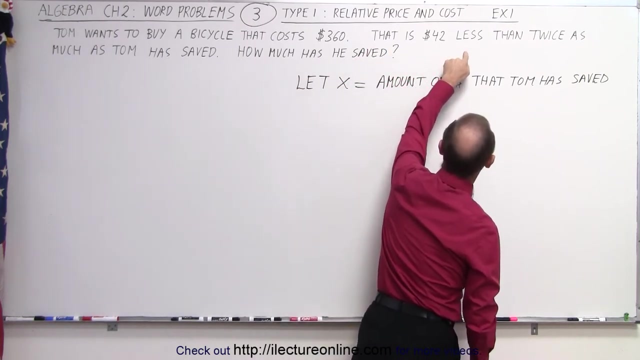 like that Just be very descriptive- what X represents. Now we need to read the sentence and let's see here We need to figure out something relative to the price. It says here that $360 is $42.. We subtract $360, we get $40, we have $42- less than twice as much money as Tom has saved. 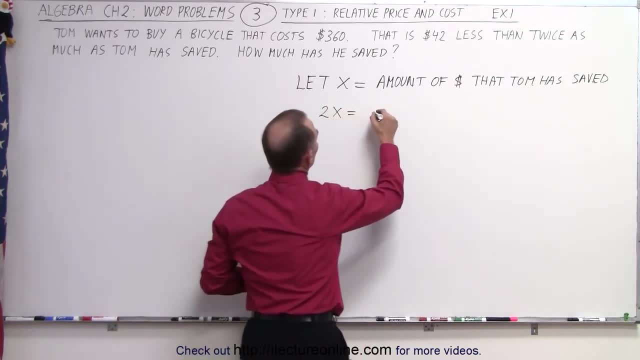 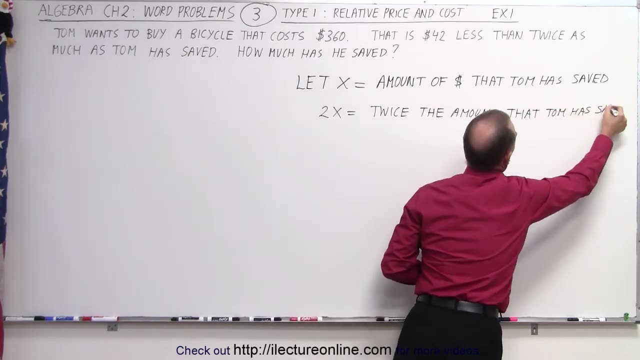 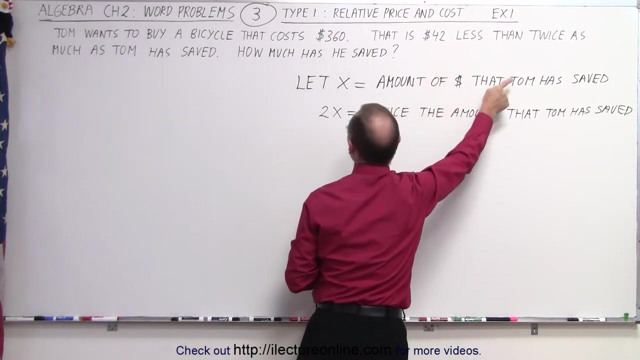 So that means that 2X is equal to twice the amount Tom has saved. Now we subtract $42 from that, we will have $42 less than twice as much Tom has saved. So 2X minus $42 is equal to $42 divided by 42.. 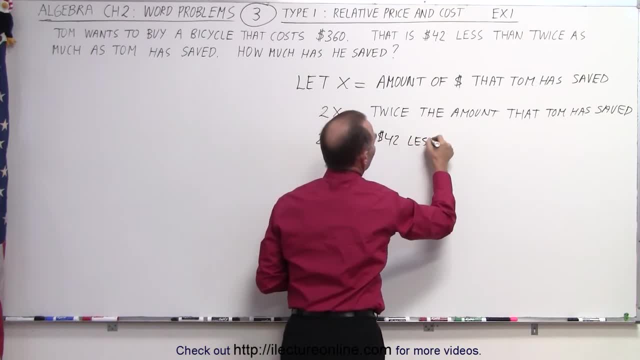 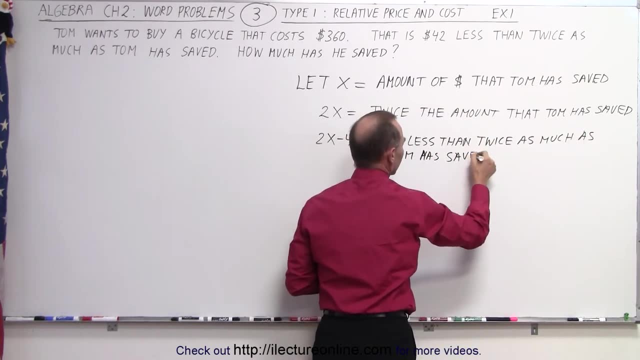 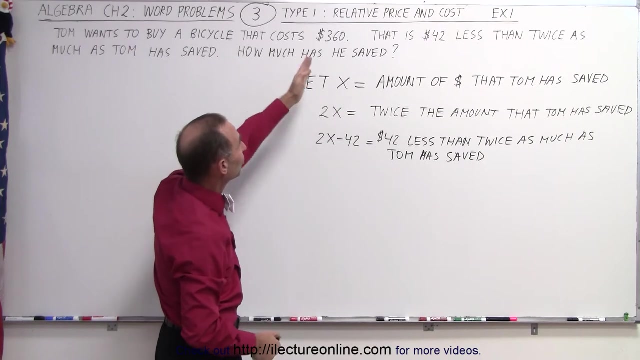 $42, less than twice as much as Tom has saved. Now notice the progression. We started with letting x equal the amount that Tom has saved. Then we realize that we're expressing the price of the bicycle in terms of $42, less than twice as much as he has saved.